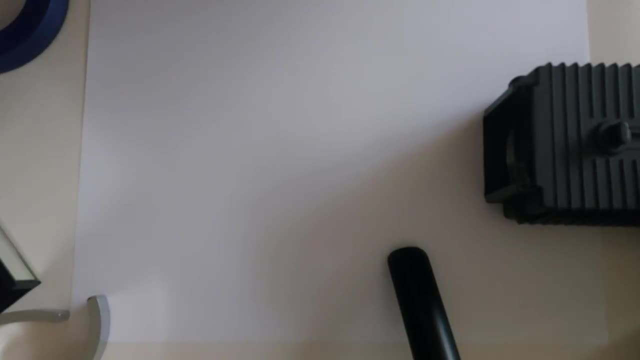 Hi everyone, and welcome back to another episode of science. In this episode, I'm going to be demonstrating the law of reflection, which states that the angle of incidence is equal to the angle of reflection, and I'll also be showing you how to measure the angle of incidence and angle of. 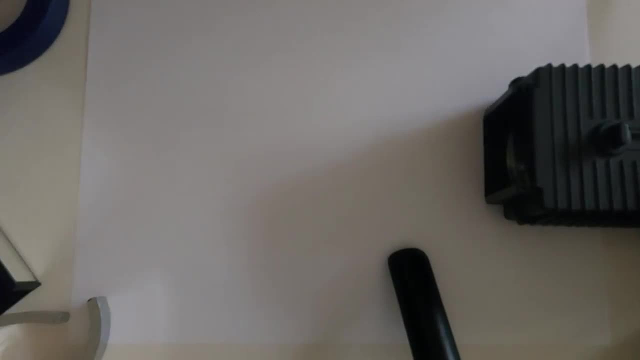 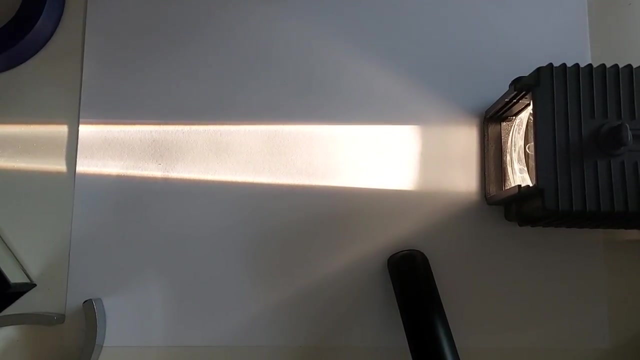 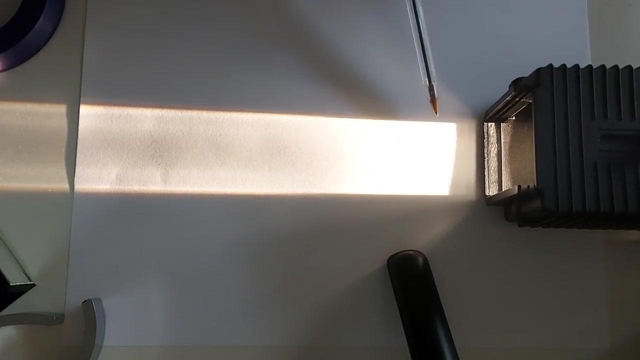 reflection With me. I've got a light box here which is connected to a power supply. I'll just turn it on and I've got 12 volts running through this light box. Now there's a lens here and I can adjust this lens in order to make this beam of light diverging or converging. I'll also need 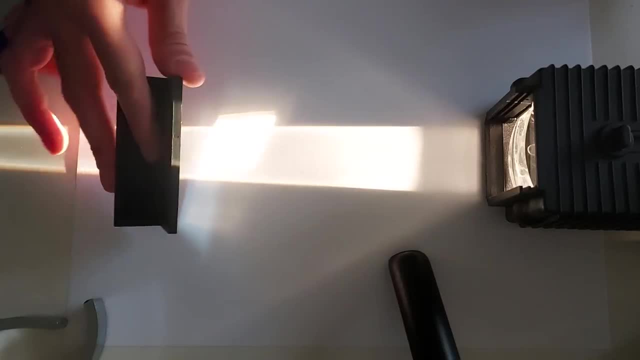 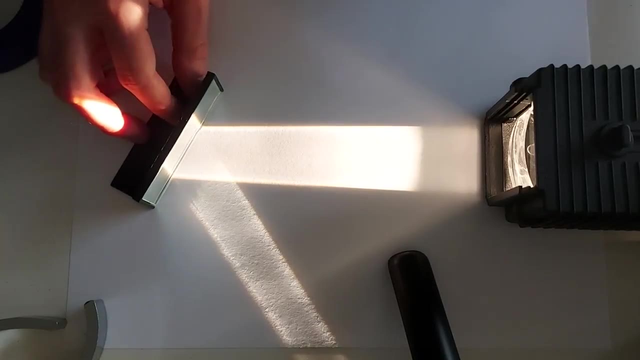 this plain mirror here, and this plain mirror obviously allows me to reflect that beam of light. Now, this beam is a little bit too wide for me, so I'm going to go ahead and measure it out and I'll just turn it off. and I've got 12 volts running through this light box. 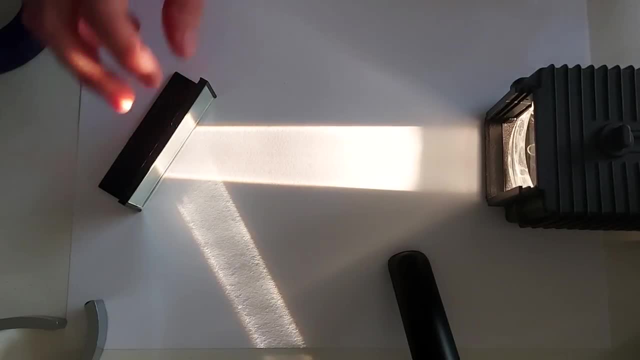 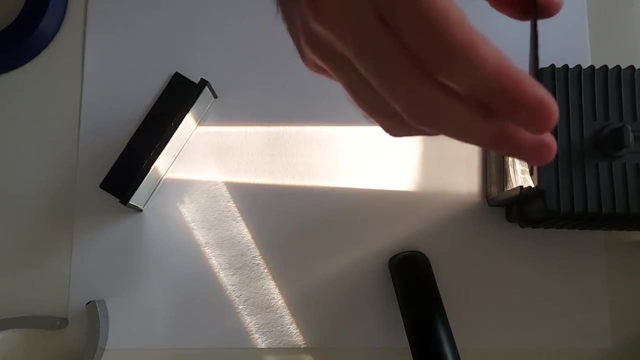 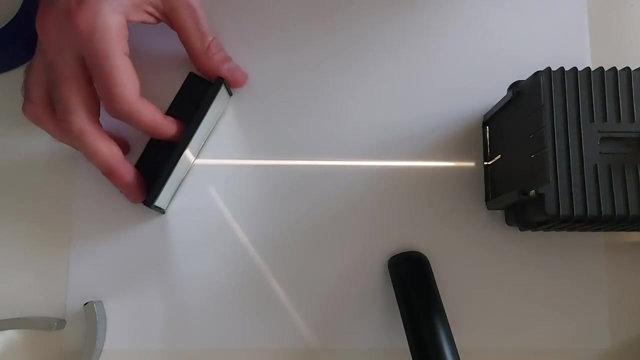 to use and accurately measure my angles. So I've got this piece of plastic here which has some really thin slits cut into it And by placing that into my light box I can make my beam of light much more narrow And therefore it's going to make measuring my angle. 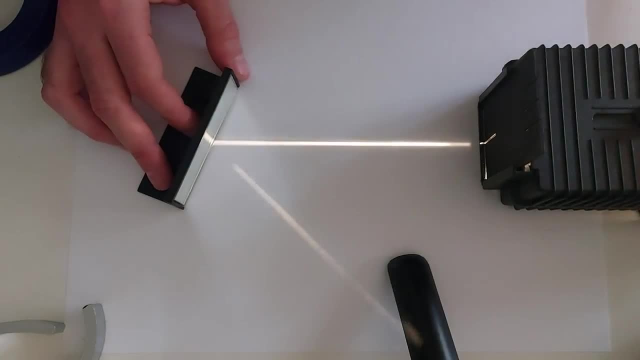 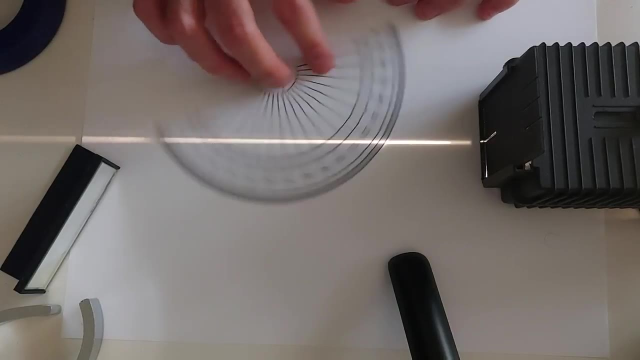 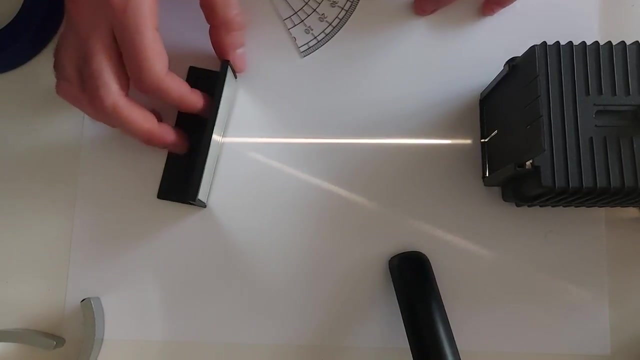 of incidence and angle of reflection much more accurate. Now, to measure those angles I'll also need a protractor, And I've just got this paper protractor here with me today. You can see as I move the mirror around that reflected ray of light. 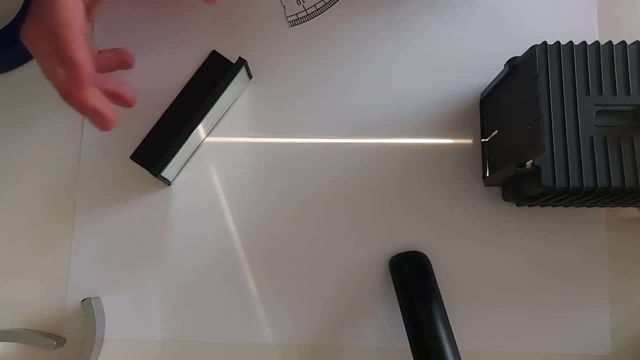 is being reflected at different angles, And that's something we can measure. The law of reflection tells us that the angle of incidence is equal to the angle of reflection, So I want to show you that, to you, today I've got my incidence ray. 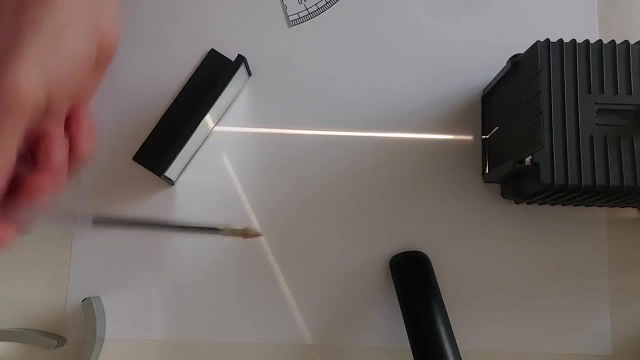 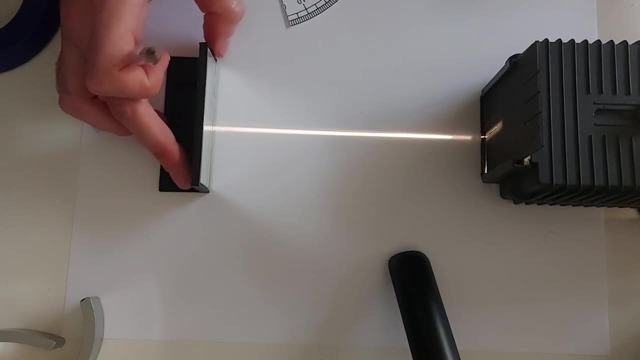 or my oncoming incoming ray of light, And this is my reflected ray of light. For now, I might just start with having the mirror perpendicular or 90 degrees to my incidence ray And, if you imagine, an imaginary line called the normal. 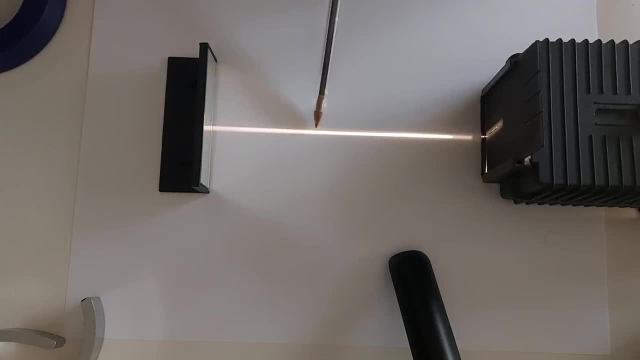 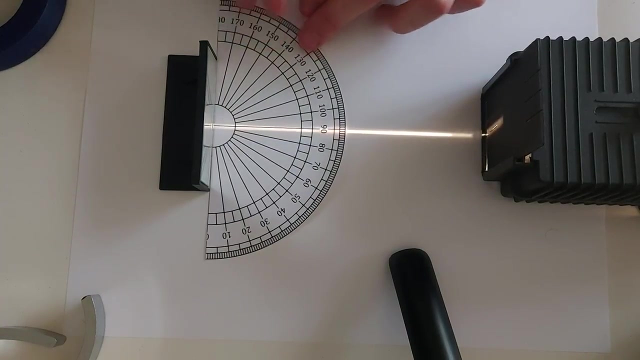 the normal is 90 degrees to the surface of the mirror. So the normal is running 90 degrees, 90 degrees, 90 degrees. And the normal is important because we measure the angles from that imaginary line, from the normal. So at the moment, the normal for this plain mirror, 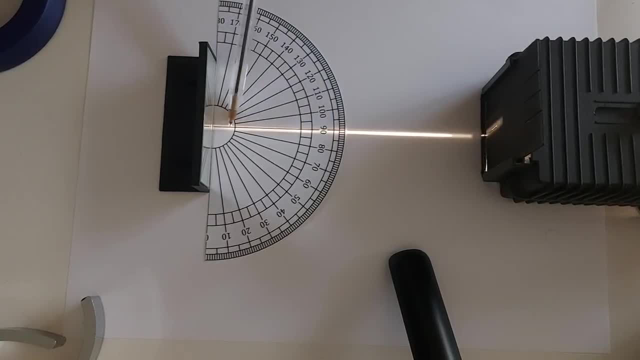 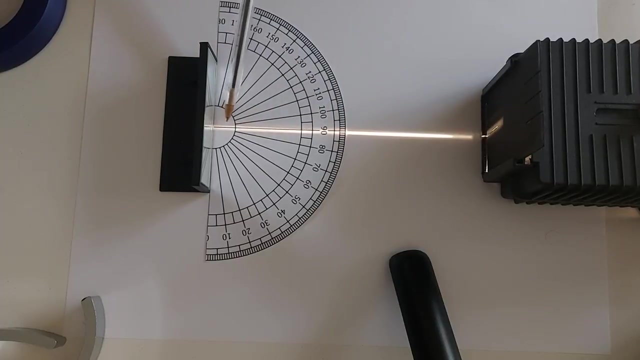 is just running along this 90 degree line here And that is the line in which we are going to measure our angles from. So at the moment, our ray of incidence, or incidence ray, is coming along the normal, hitting the plain mirror. 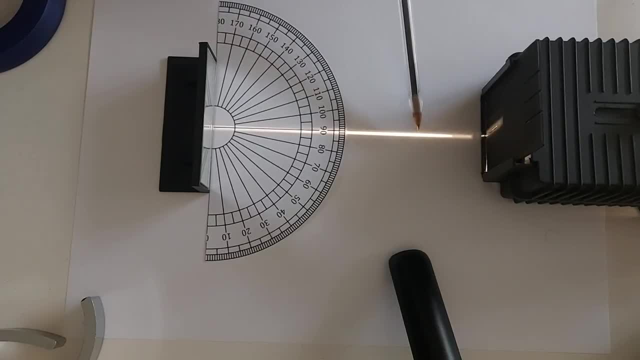 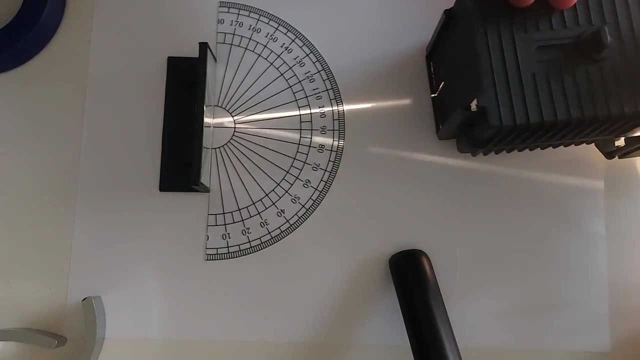 and being reflected back out along the normal. So in this case, my angle of incidence is actually zero degrees And therefore my angle of reflection is zero degrees as well. But what happens if I move this light ray, or light box, I should say? 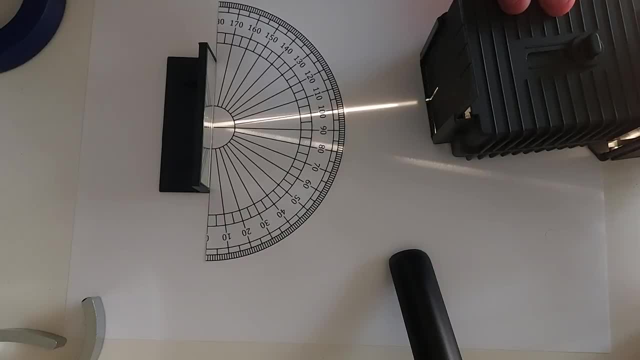 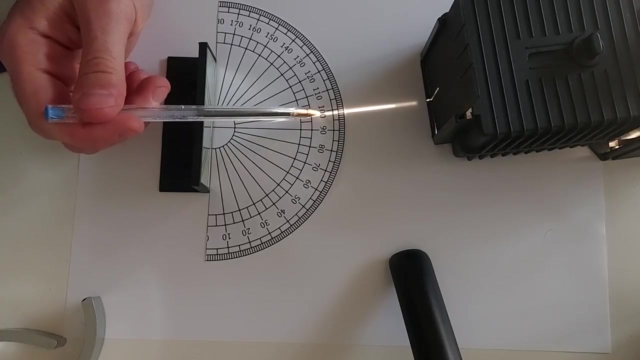 and a little bit tricky to get it exact. Okay, I think that's about good enough. So in this case I've moved my incidence ray 10 degrees outward, 10 degrees outward. So now my angle of incidence is 10 degrees. 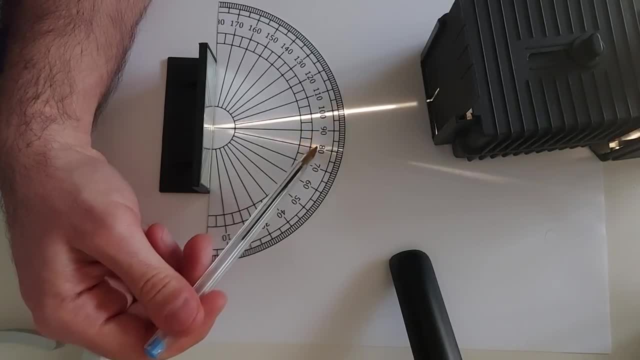 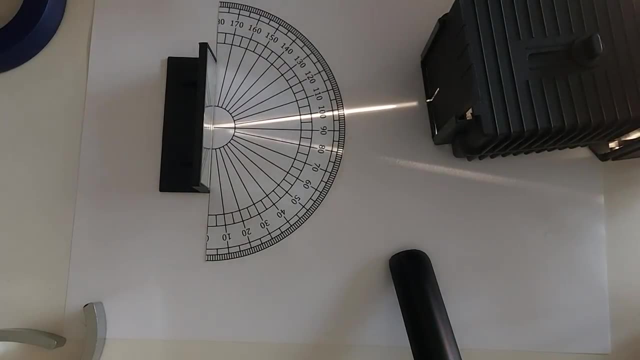 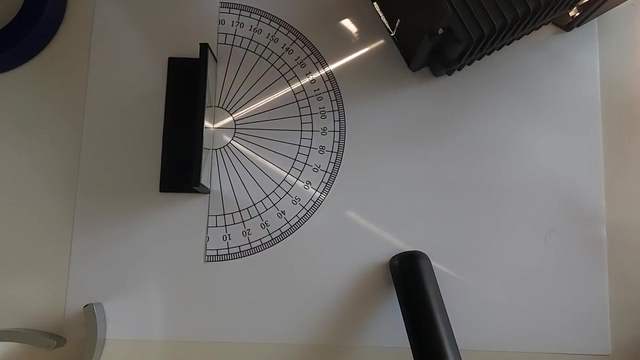 And if I look at my angle of reflection, that's also now 10 degrees as well. So my law of reflection is being obeyed. Let's try a couple more angles. Let's bring it out here. Just try to line that up as best I can. 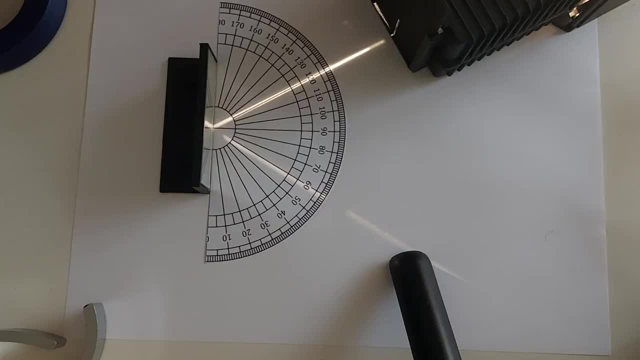 It may not be perfect. just because you know I'm using a printout paper protractor, It's difficult to line it exactly along the line. Maybe the plain mirror is even not exactly flat, But we can get close enough to observe the law. 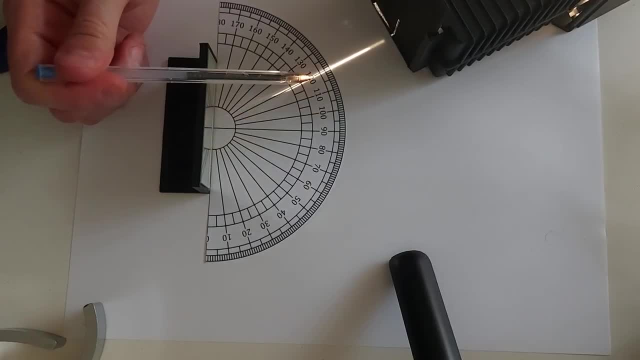 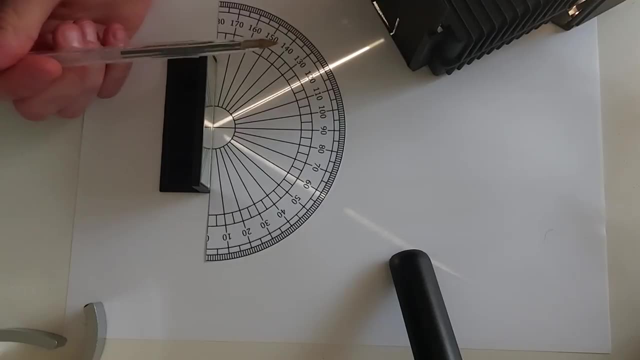 So in this case, I've got 10,, 20, 30 degrees for my angle of incidence, And for my angle of reflection I've got 10, 20, 30 degrees as well. So my law of reflection is being obeyed. 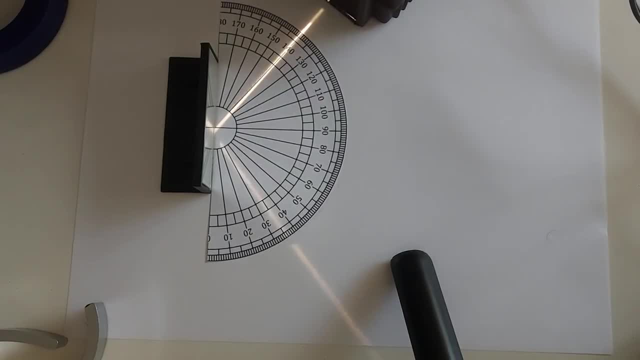 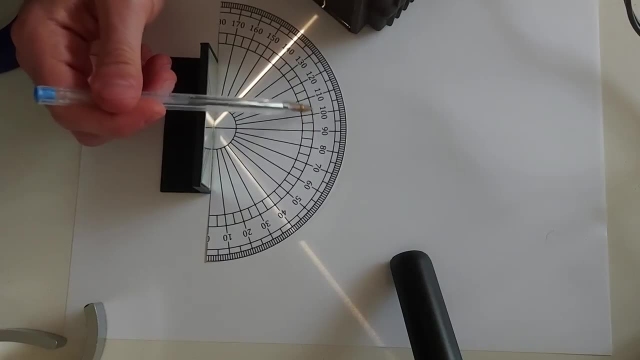 Let's do a couple more. I'll go wider this time, Just try to line it up as best I can. Okay, so from the normal I've got 10,, 20,, 30,, 40,, 50 degrees. 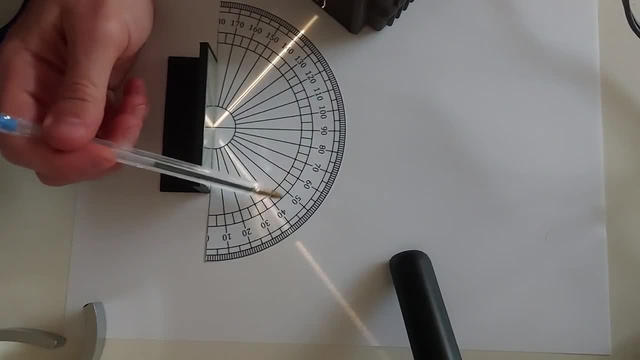 And my angle of reflection 10,, 20,, 30,, 40, 50 degrees as well. You can see it's just a little bit more, but that's only because I probably haven't lined it up exactly perfectly. Let's go really wide now. 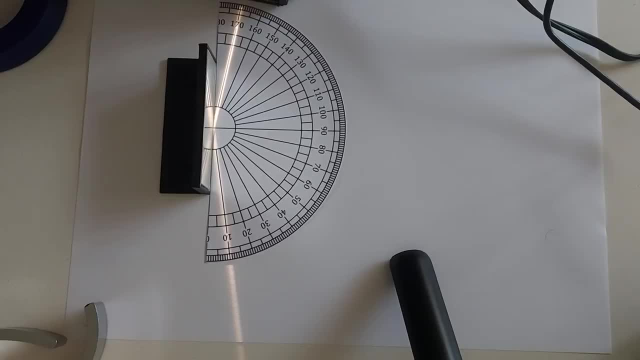 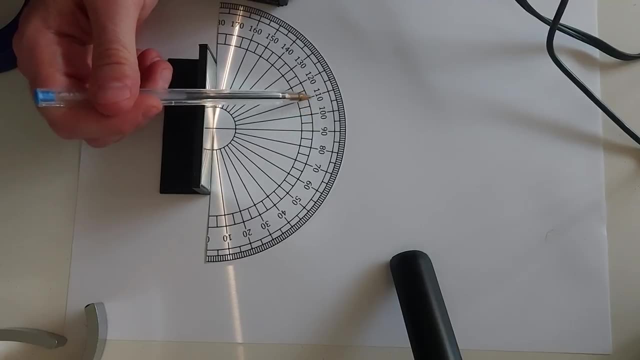 Let's come all the way here And count again. from the normal, which is from this 90 degree line, I've got 10,, 20,, 30,, 40,, 50,, 60,, 70,, 80 degrees. 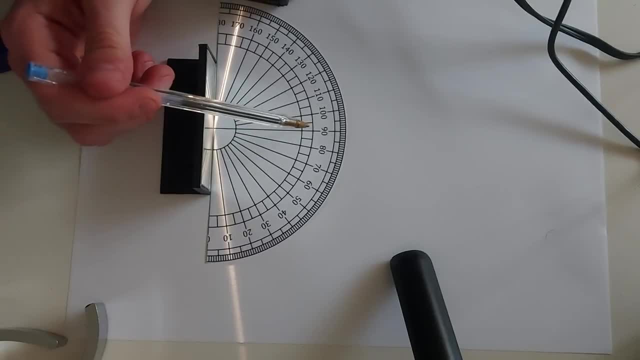 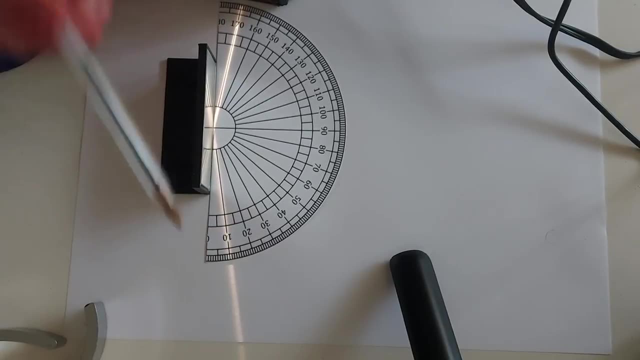 as my angle of incidence And my angle of reflection is 10,, 20,, 30,, 40,, 50,, 60,, 70, 80 degrees as well. So in all cases, in all examples, my law of reflection is being obeyed, which is great. 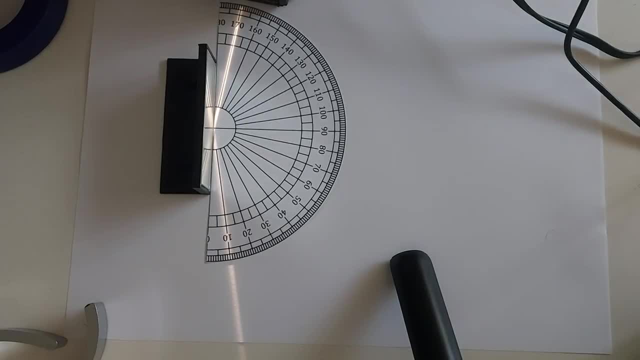 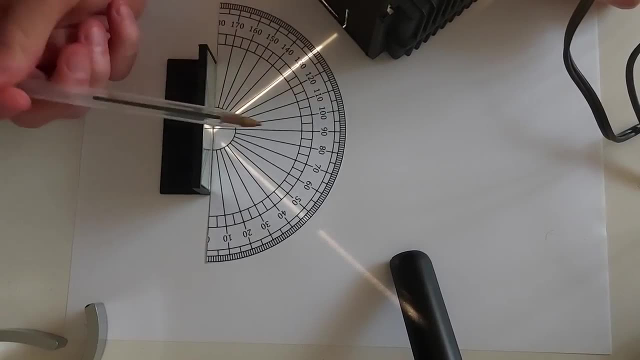 And that is also how you measure the angle of incidence and angle of reflection. You need to measure the angle from the normal, which is an imaginary line running 90 degrees to the surface. And that's what we're going to do: We're going to use the curve mirror. 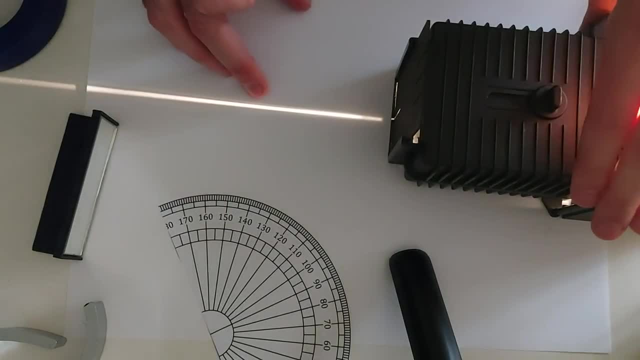 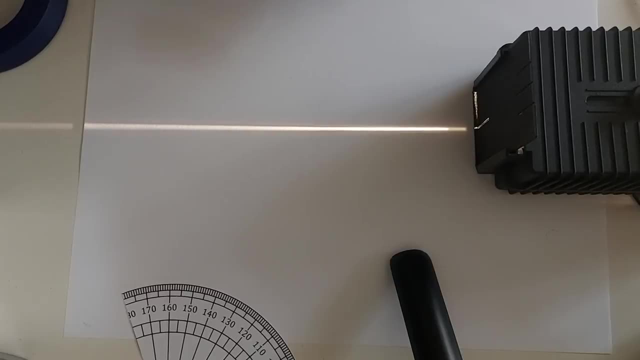 And I'm using that curve mirror to measure the angle of incidence of my plane mirror. Now we can also use curved mirrors as well to make the light bounce in interesting ways. Let me just adjust my materials here. Okay. So I've got here a curved mirror. 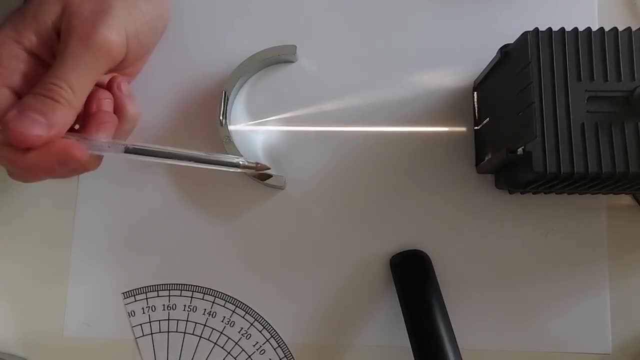 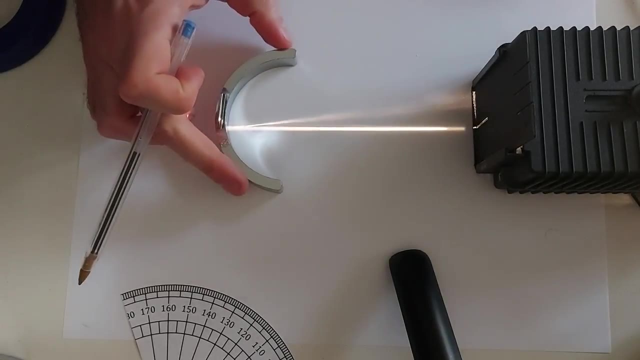 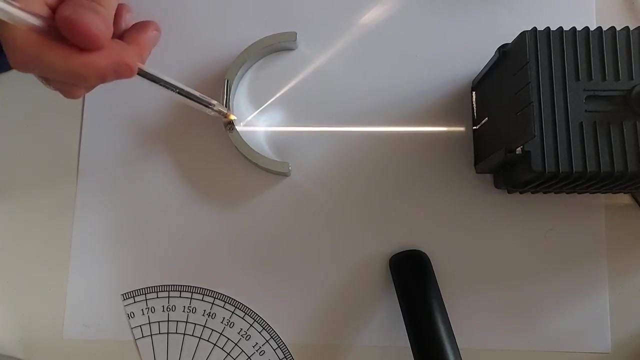 And right now I'm using the concave side of the mirror. You can kind of imagine like going into a cave, So it's curved inwards And so we say that it's the concave side, okay side. and you can see as i move the mirror up and down, the instance ray is hitting a different angle. 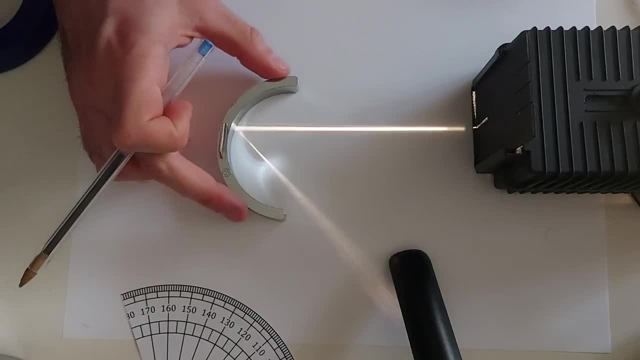 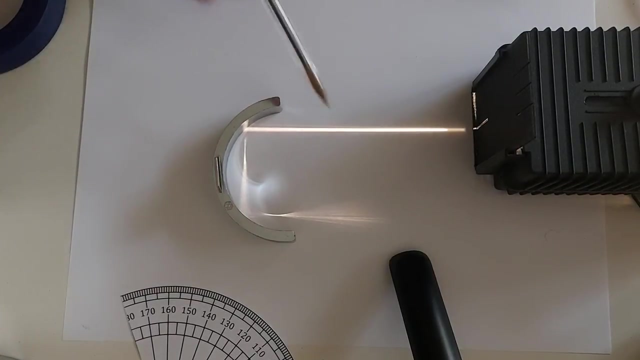 from within the mirror, which makes the reflected ray reflect at different angles, and i can even make this cool triangle shape as well, or i can actually make a square shape as well, so i can make the light rays bounce at right angles. light always travels through space in a straight line.